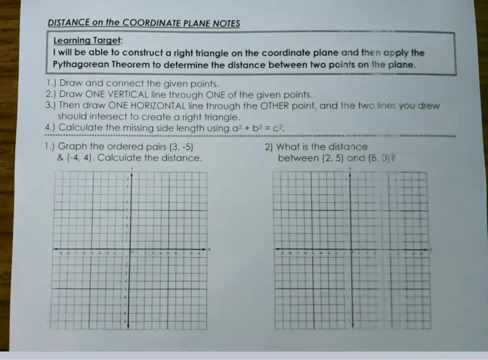 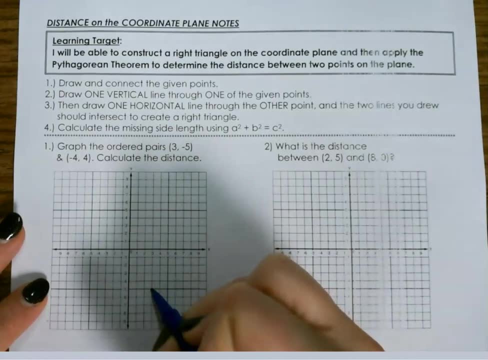 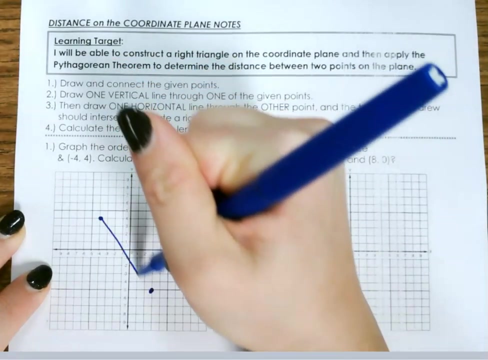 we calculate the missing side using a squared plus b squared equals c squared, the Pythagorean Theorem. So our first example: we're going to plot 3, negative 5, and negative 4, 4.. Then we're going to connect those points, Then we're going to draw a vertical line. 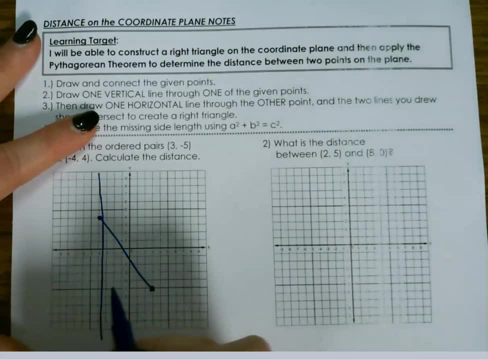 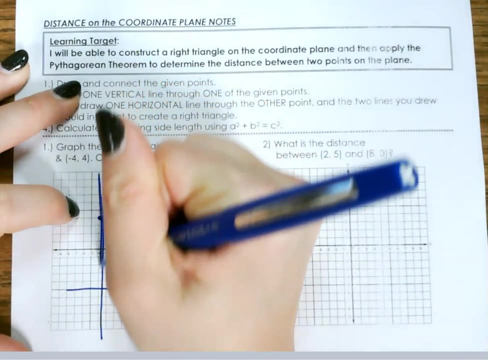 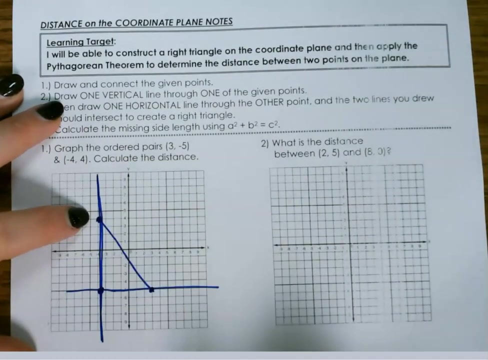 through one, assuming that's a straight line, and a horizontal line through the other. So for our first one, we now calculate the distance from the coordinate plane to the other, So between where they intersected. okay, so the way that I do this, this one is at: 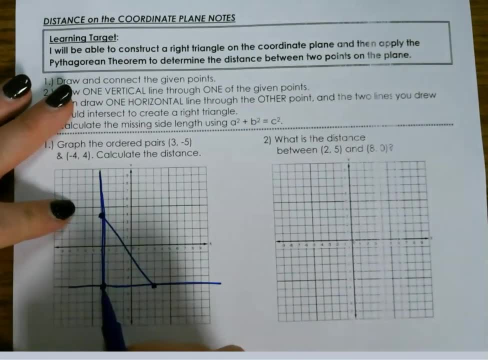 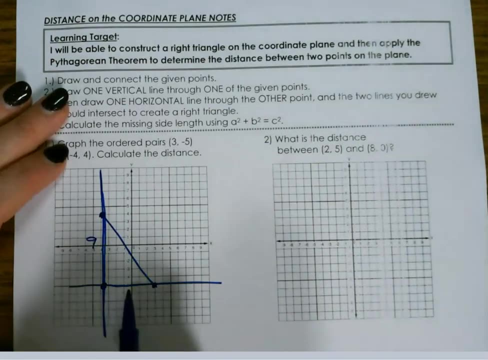 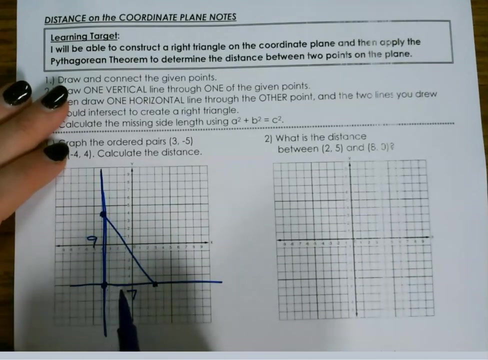 four and this one is at five. so four plus five it's going to give me nine. you could also count each individual box. this one over here is that negative four and this one is at three. so four plus three is seven. again, you could go through and count one, two, three, four, five, six, seven to get your boxes. so then, 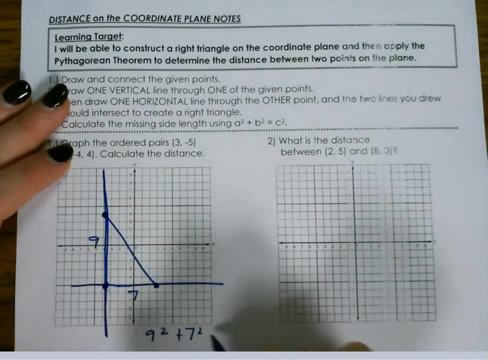 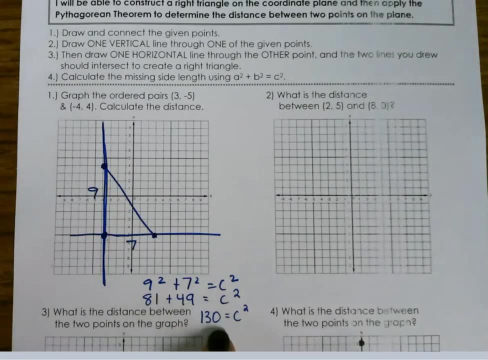 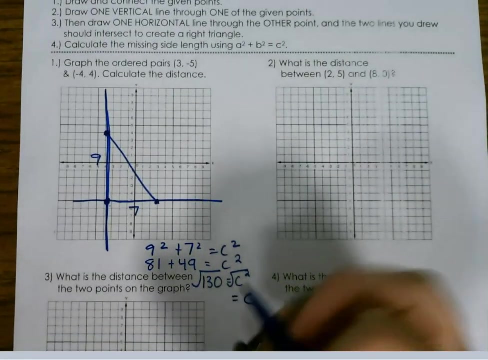 we just use a squared plus B squared equals C squared to calculate for C. so that would be 81 plus 49, which is 130. when we do the square root of this. 130 is not a perfect square, so it's going to give us a decimal of approximately 11.4. 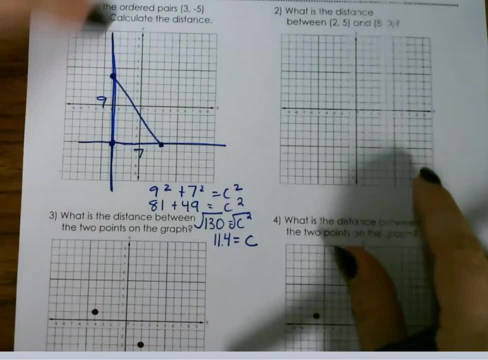 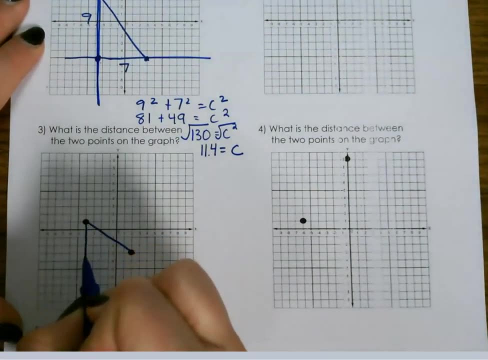 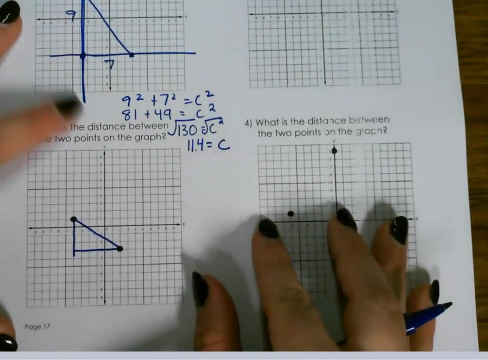 for our next example, we have our points already drawn on the graph for us, so we're going to connect them and I'm going to do a vertical line and a horizontal line. I don't always do them where they continue like this once I get the hang of what I'm doing, so here I 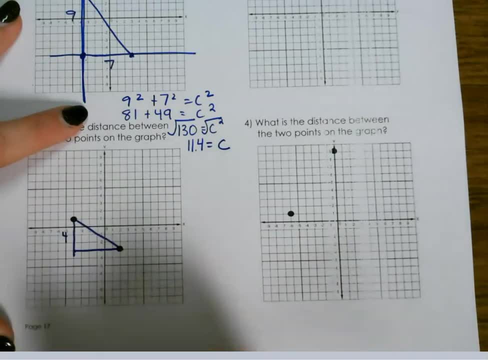 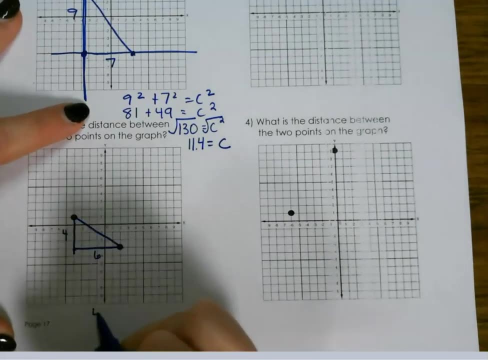 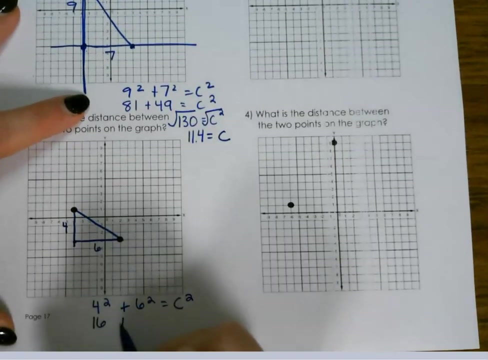 have a point at one, this one's at three, so that would be a distance of four. this one would be at negative four and two, which would be a distance of six. so a squared plus B squared equals C squared. so 16 plus 36 equals C squared. so that's.